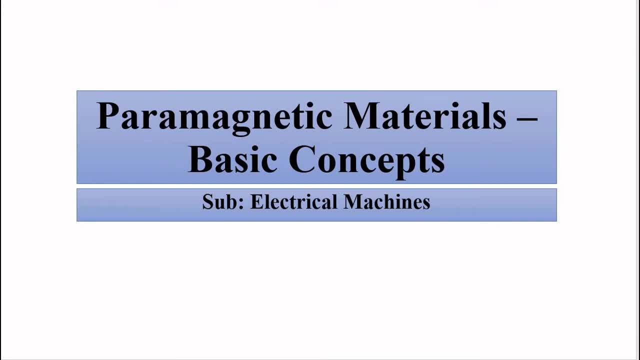 Hello friends, welcome to engineering tutorial. So we will continue our discussion related to basic concepts related to electrical machines. So in the previous video we discussed about magnetic materials and the classification of magnetic materials and we discussed specifically about the diamagnetic materials. So in this video we are going to discuss about 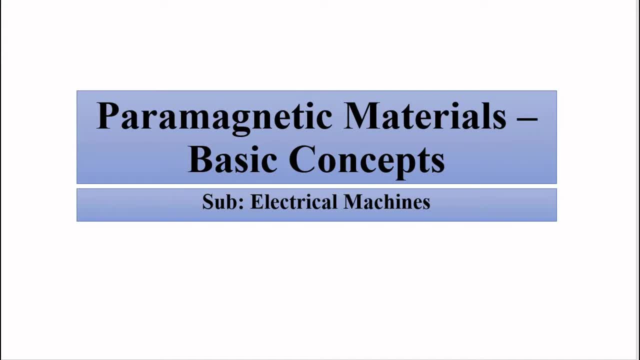 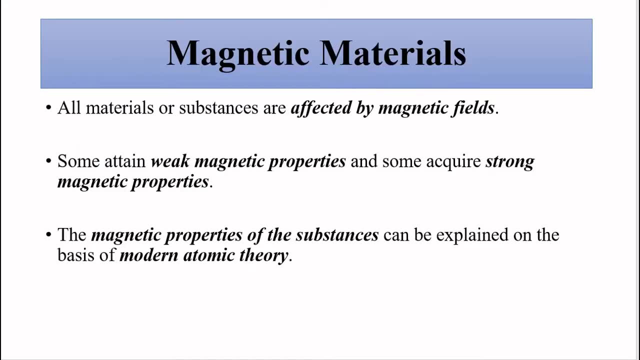 the paramagnetic materials. So just a quick recap. So we know that every object or material, they are affected by magnetic fields. So when an object is placed in a magnetic field, because of the influence of the magnetic field it can attain magnetic properties. So 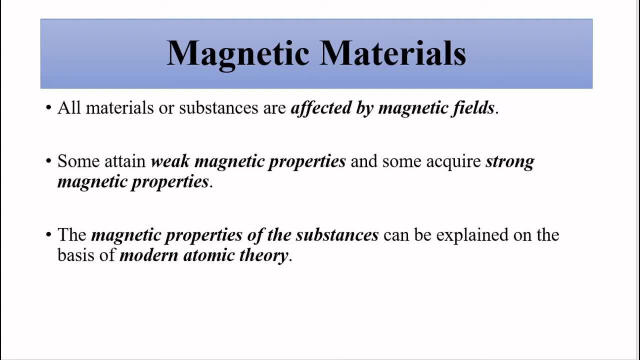 to which extent it acquires magnetic properties, how strong or how weak it is. it depends on certain properties, The important properties related to magnetism which we have discussed: magnetic flux density, magnetic permeability, magnetic susceptibility, intensity of magnetization, magnetic intensity. all that we have discussed, So you can check that. 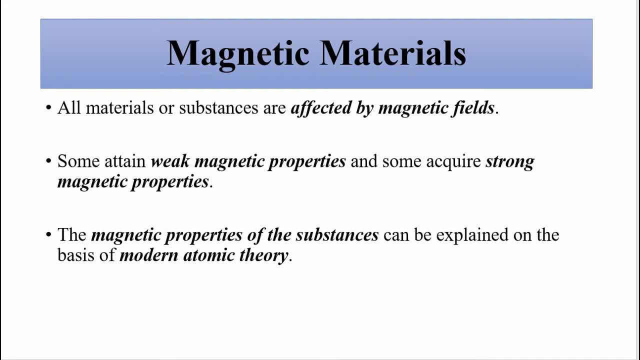 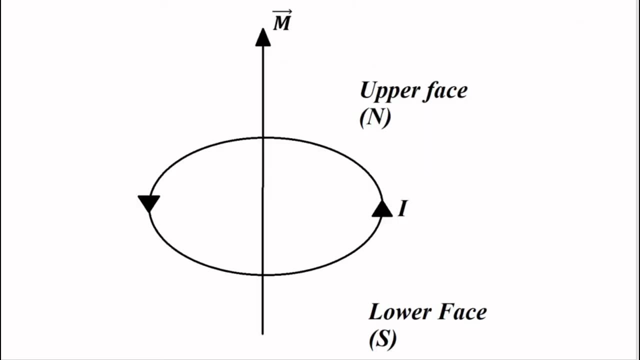 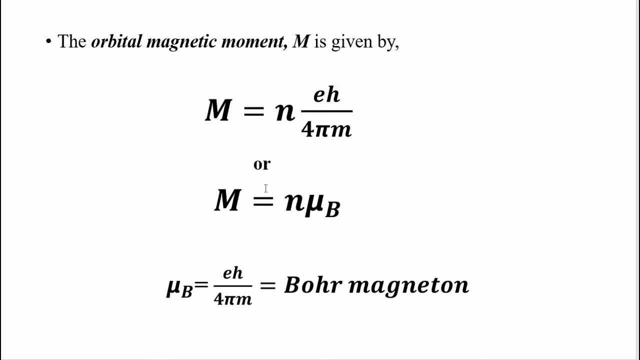 video first, then the other videos. So this magnetic property of the substance is because of the orbital movement of electrons, which behaves like a current loop and that behaves as a magnetic dipole, with the orbital magnetic dipole movement given by this. We have already covered it. So the classification of 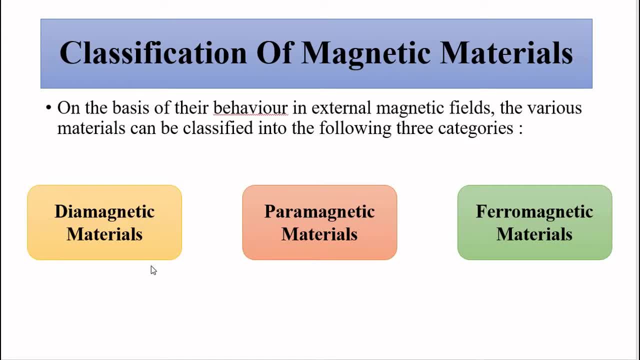 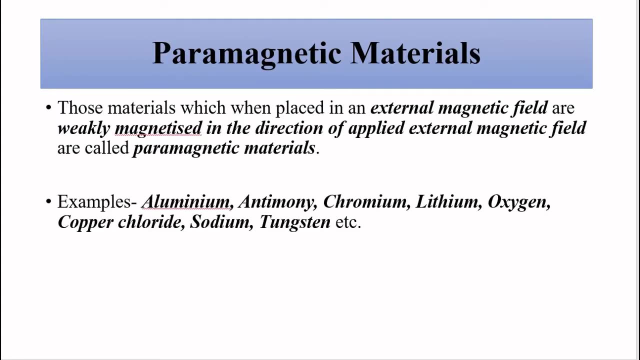 magnetic materials is into three categories: diamagnetic, paramagnetic and ferromagnetic materials. Diamagnetic: we have covered In this video. we are going to discuss about paramagnetic materials. So paramagnetic material is one. when it is placed an external magnetic field, it is weekly magnetized in the direction of the applied external field. So 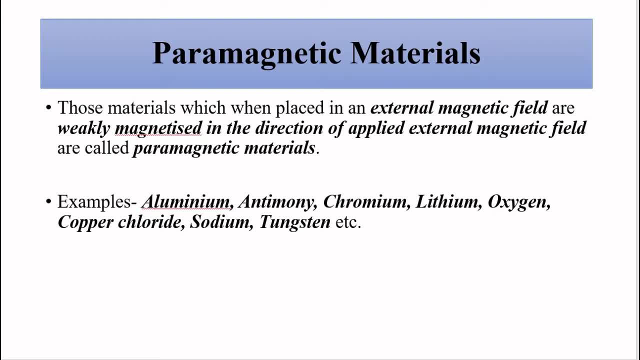 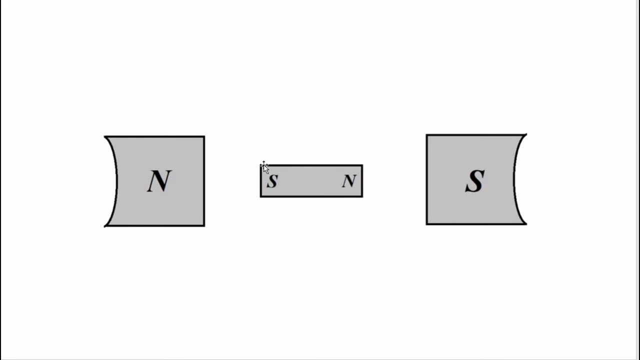 in diamagnetic it was weakly magnetized in the opposite direction. Here it is in the direction. So let us say we have a material, let us say this one: the middle, it is placed in the magnetic field. It is magnetized in such a way that the opposite extreme ends of the material they acquire. 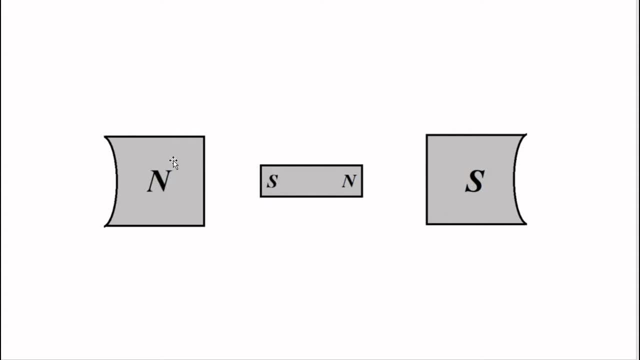 opposite polarities with respect to the polarity of the magnetic field in which it is placed. So it means that the end which is towards the north pole of the magnetic field- external magnetic field- that will acquire south pole, it will become south pole opposite, and the one which is facing the south pole of the external field, that will become north pole. 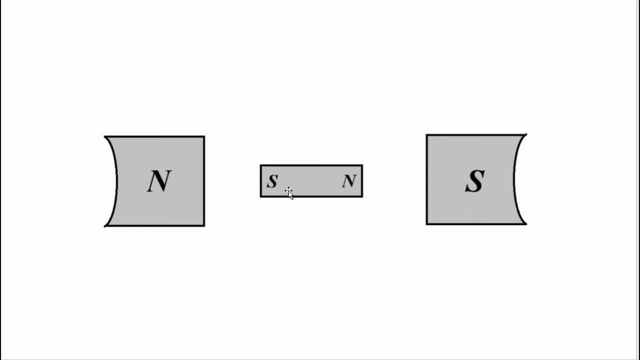 So here, as opposite to the diamagnetic materials, the object, it will get attracted towards the external field, not repelled. In case of diamagnetic it was getting repelled weakly, yes, but repelled here, same weak intensity, less intensity, but it is getting attracted opposite. 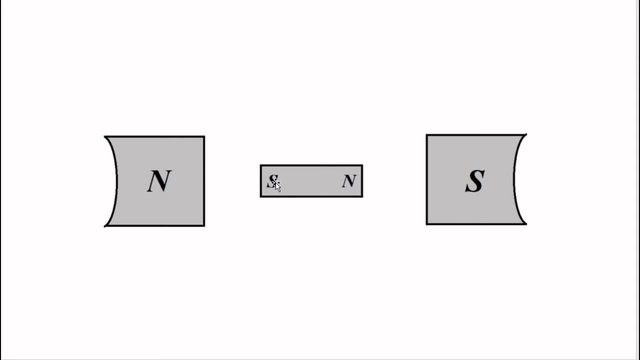 So that is the basic difference between diamagnetic and paramagnetic. In diamagnetic it was getting weakly repelled. In case of diamagnetic, north facing end acquires north pole, south facing end acquires south pole. Like poles repel each other. that is why it was getting repelled. 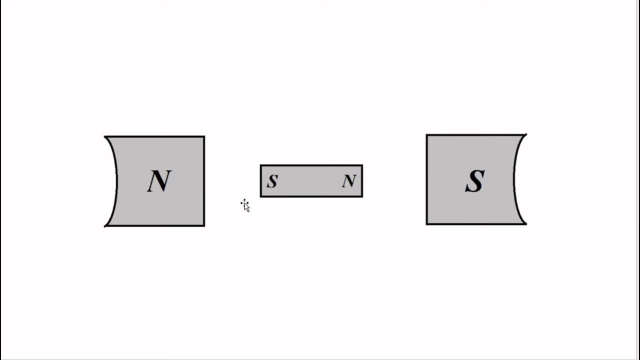 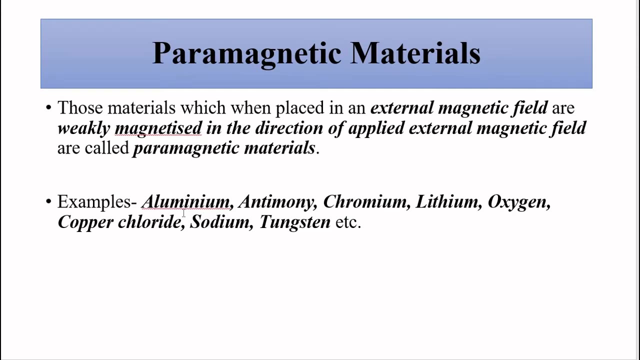 In case of paramagnetic, it acquire opposite poles: north facing acquires south, south facing acquires north. that is why it gets attracted, but weakly. the intensity is not great. Examples of paramagnetic materials are aluminum, antimony, chromium, lithium, oxygen, copper. 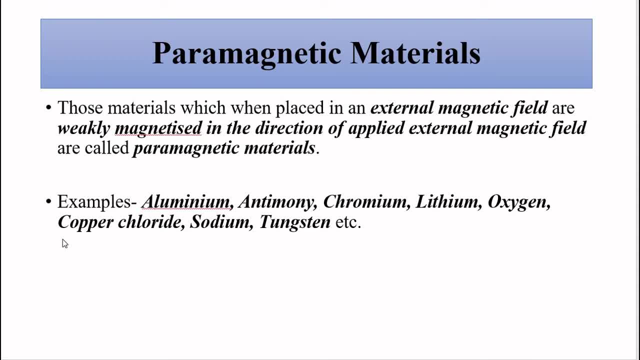 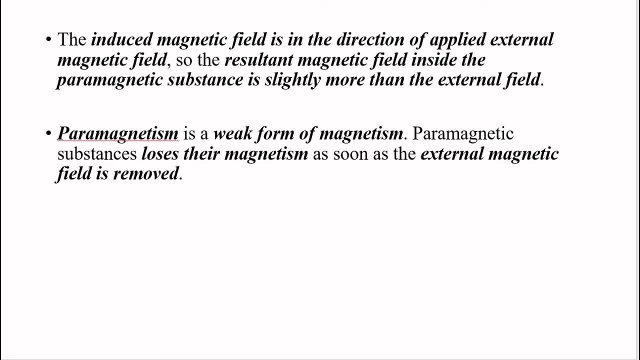 chloride, sodium, tungsten, To name a few. Now the magnetic field which gets induced in the direction inside this material is weak. It is of weak intensity, So similar to diamagnetism, these paramagnetic materials, they lose their magnetic characteristics whatever feature they acquire. 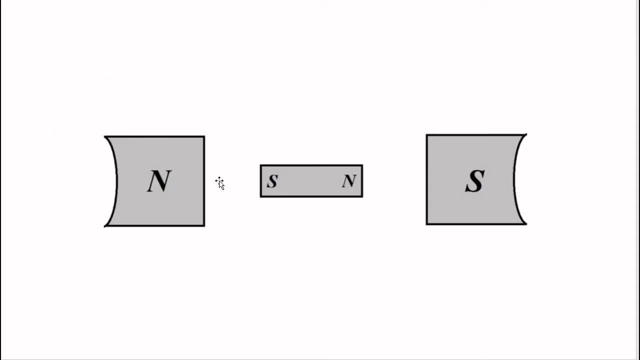 As soon as this external field gets induced, So the magnetic field which gets induced in the direction inside this material is weak. It is of weak intensity, So similar to diamagnetism, these paramagnetic materials. they lose their magnetic properties, They do not retain it. 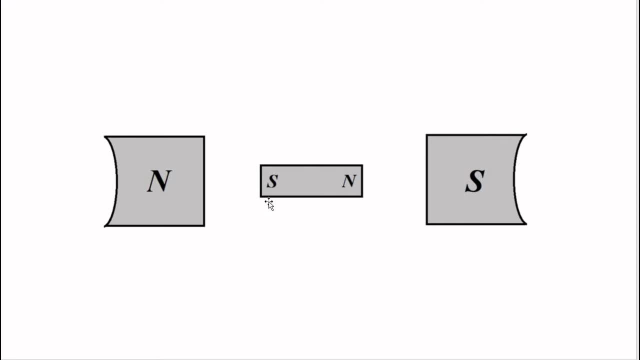 In case of diamagnetism also, that repelling nature, it loses that behavior as soon as this magnetic field is removed or it is taken away from this magnetic field. So in both diamagnetic and paramagnetic, one thing is common is that they lose their magnetic 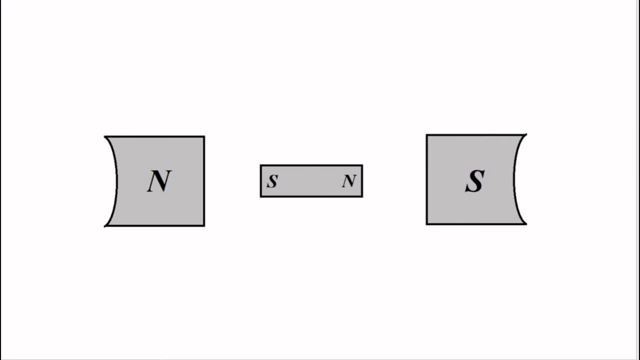 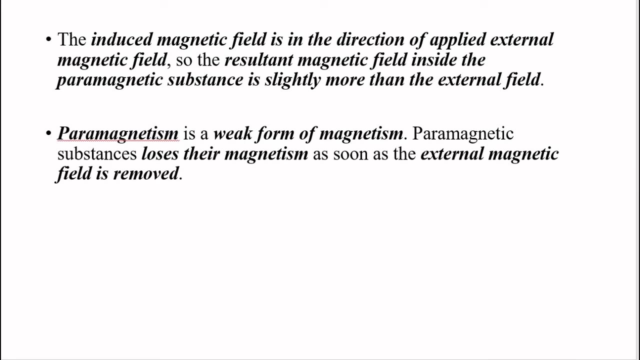 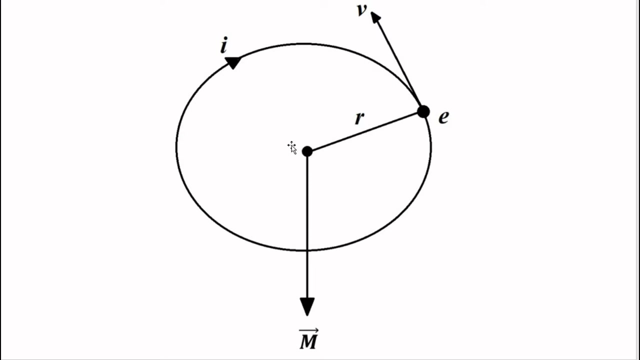 behavior, the induced magnetic behavior or the forced magnetic behavior, as long as the external magnetic field is removed. Now, what is the cause of paramagnetism? Now, in case of diamagnetism, we know that whatever magnetic property, material or a substance has, it is because of the magnetic dipole movement, because of the orbital motion of the electrons. 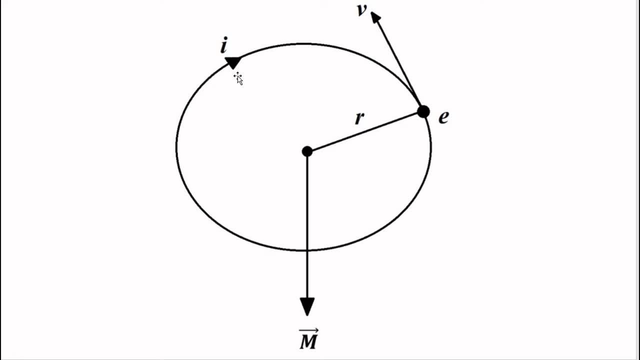 which constitutes an orbital current in the opposite direction and that current loop. it behaves as a magnetic dipole and that dipole movement, the orbital magnetic dipole movement, is responsible for the magnetic behavior. In case of diamagnetic materials, the magnetic dipole movements used to cancel each other. 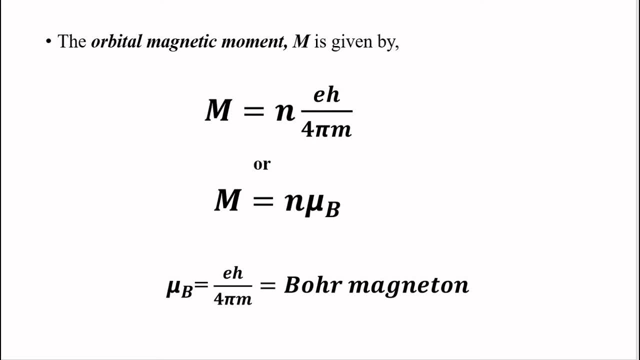 out. They existed in pairs: Dimensional magnitude, opposite direction, no net dipole movement. that's why weak magnetic behavior, repelling type magnetic behavior. But in case of paramagnetism, even though the characteristics are weak, the magnetic characteristics are weak but they attract the magnetic lines of force because they get magnetized in the 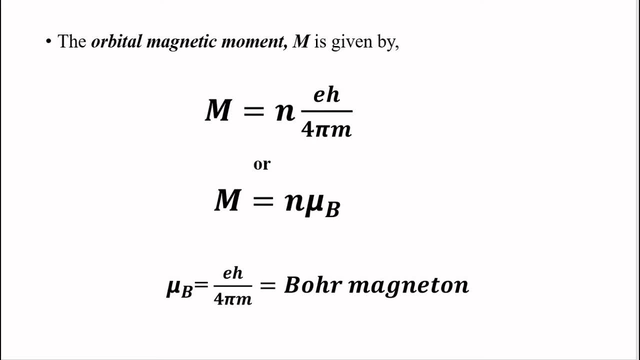 direction. Now, what is the reason behind that? is that when a paramagnetic material is without the influence of the external magnetic field, when it is away from a external magnetic field, the orbital magnetic dipole movements. because of the revolving electrons, they are randomly aligned in random directions. 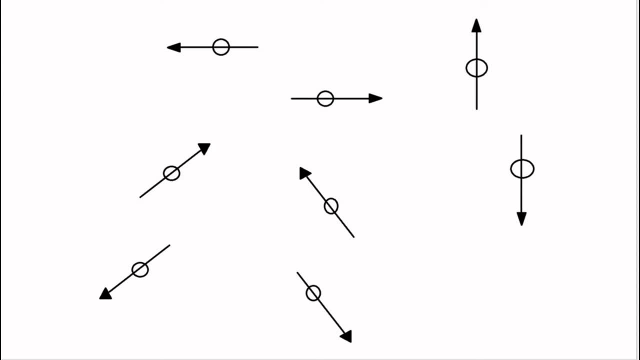 But when it is placed in an external magnetic field They get magnetized, get aligned in the direction of the magnetic field, in one direction. So the net resultant of all these orbital magnetic dipole moments, because of the orbiting electrons, that constitutes a non-zero dipole moment. The magnitude is very less. yes, the magnitude is very. 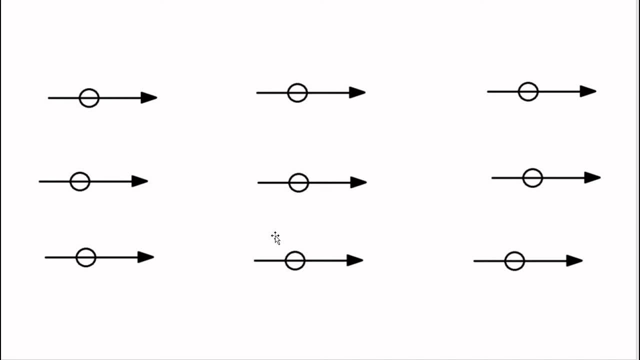 less, but it is greater than 0, less but greater than 0, and because of that paramagnetic material acquires this kind of a characteristics: opposite ends of the extreme ends of the paramagnetic material. they acquire opposite polarities with respect to the polarity of the magnetic field. 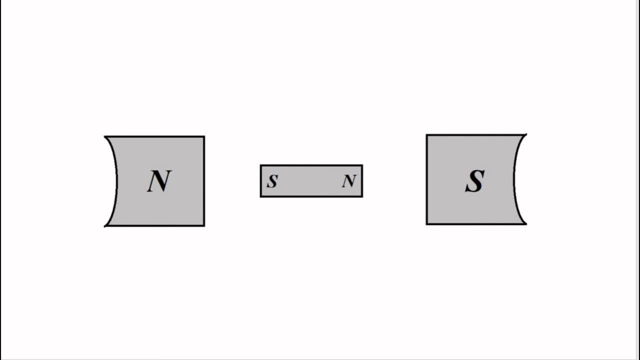 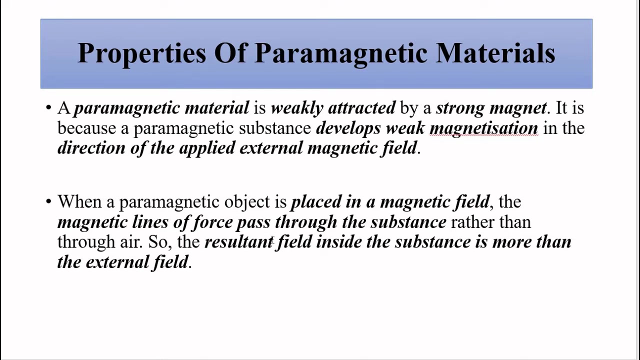 in which it is placed. So there are some properties of paramagnetic materials which are important, like we discussed in diamagnetic cases. Paramagnetic material, in the paramagnetic material, the magnetism which is induced, it is weak and this kind of attractive type, so it is weakly attracted by 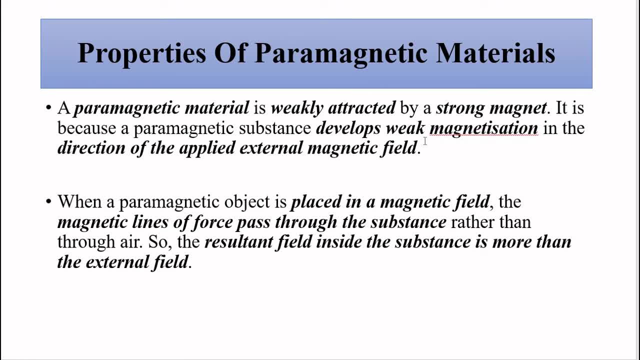 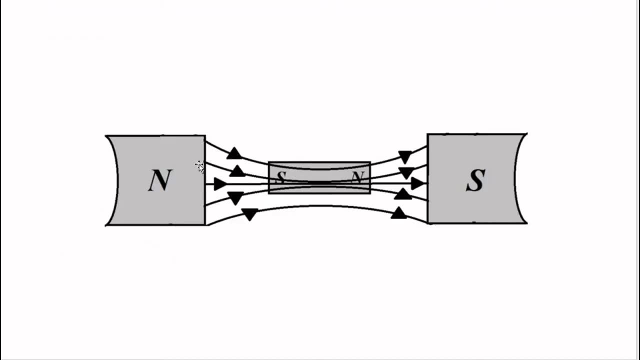 a strong magnet because of the weak magnetization, attractive type magnetization, which is developed in the direction of the applied magnetic field. When a paramagnetic material is placed in an external magnetic field, the magnetic lines of force, they move into the material through the material. but 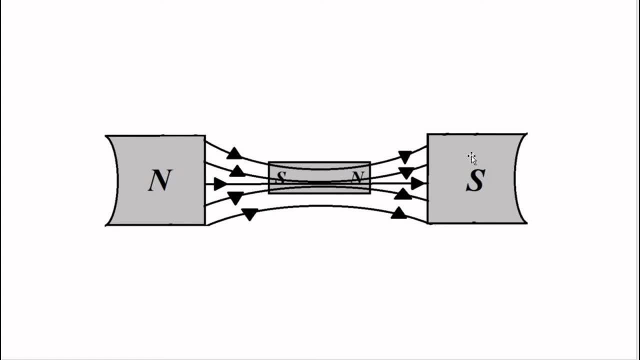 in case of diamagnetic, they moved away from the material, passed away from the material. they did not crowd into the this paramagnetic material. So we can say that the magnetic field is placed in the magnetic field and the brazil Battlesky. as you can see that, even though the magnetic 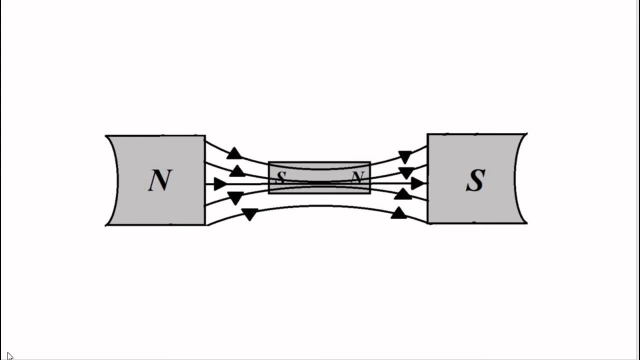 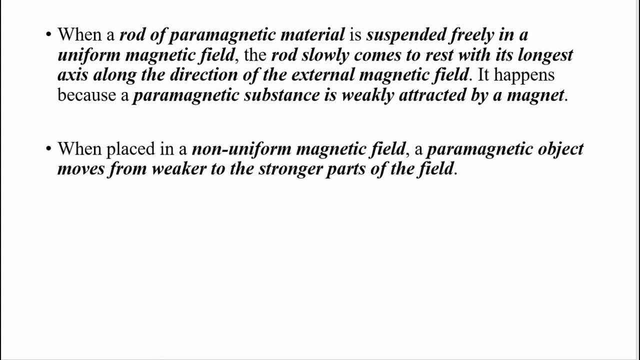 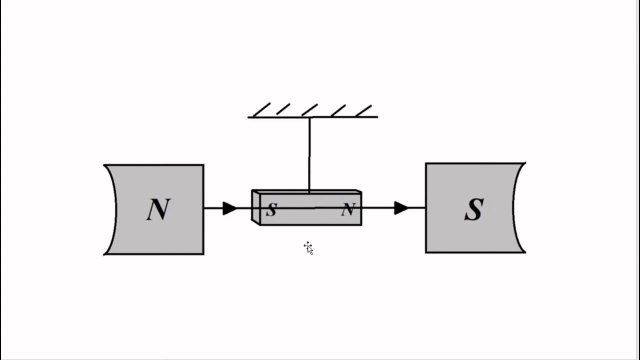 characteristics are weak, they are attractive type. that's why the magnetic lines of force they allowed to pass through the paramagnetic material. next, when the paramagnetic material, it is placed in a an external magnetic field, It aligns itself In the direction of the magnetic field. why? because opposite poles, they attract each other, north attract. 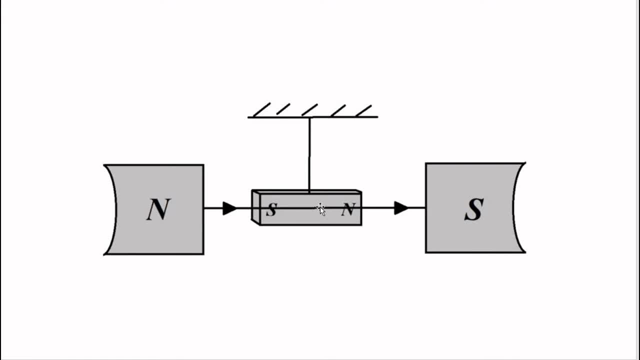 south, south attracts north. so that's why it gets aligned with its longest axis in the direction parallel to the magnetic field, external magnetic field. but in case of diamagnetic the longest axis was perpendicular. ok, it was perpendicular because in that case it used to repel. this was north, this was south, north, north, repel, south, south. it used to repel. but 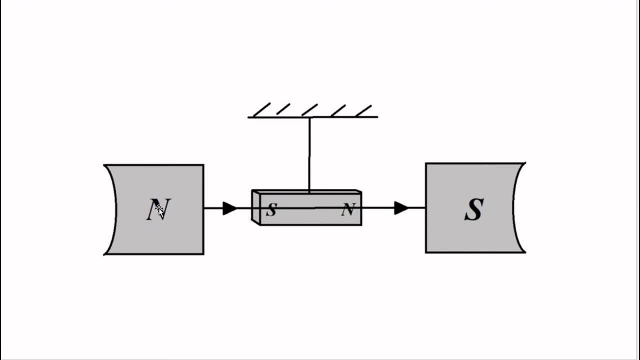 in this case it is attractive type. so north attracts south, south attracts north, so it's always its longest. axis is parallel to the external magnetic field. then the other important characteristics, that is, The permeability or the relative permeability of the paramagnetic material or substance. 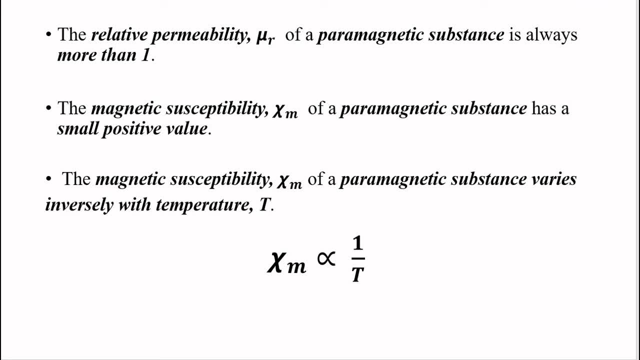 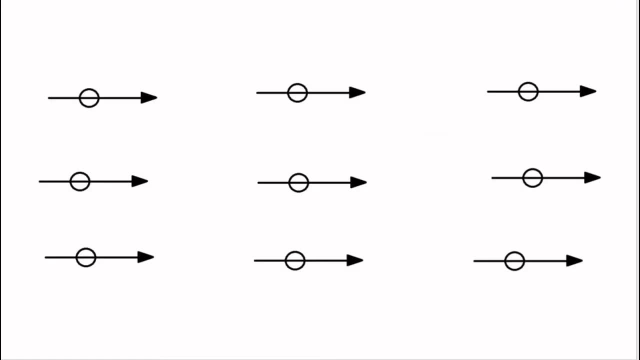 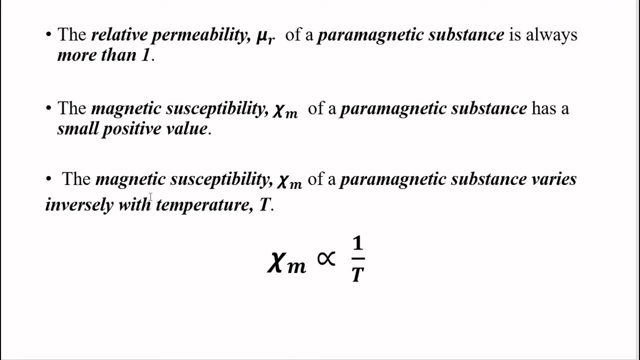 is more than one, which explains why it acquires attractive type magnetic behavior because of the non-zero orbital magnetic dipole moment. it is just greater than one, not it does not have a very high value, it just greater than one, not very high value as compared to diamagnetic. 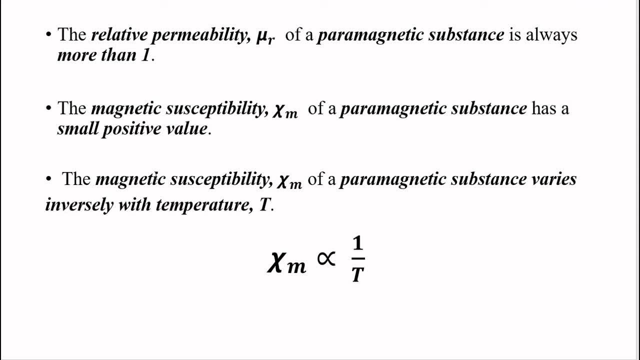 it was just less than 1 in case of diamagnetic. just less than 1. that's why diamagnetic used to used to get weakly repelled, because it was just less than 1, just less than 1, so weakly repelled it is. 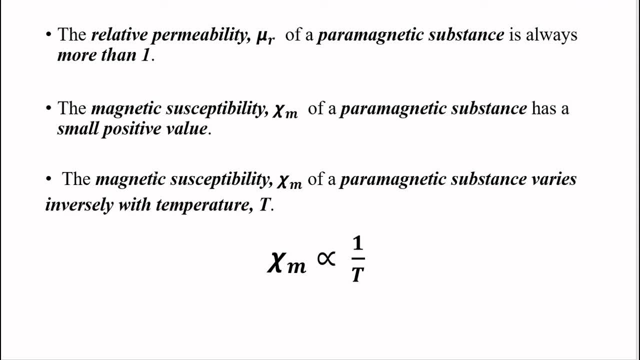 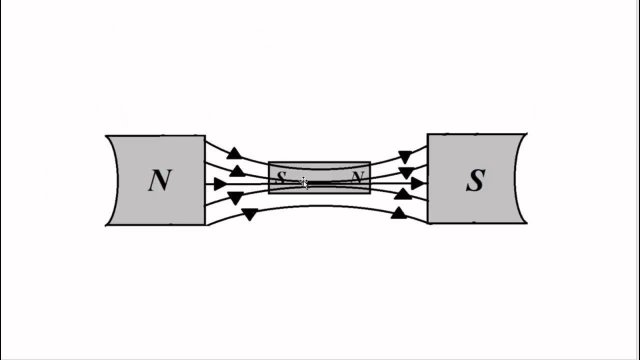 just more than 1. that's why weakly attracted the permeability. so the conductivity for magnetic lines of force is greater in case of paramagnetic material, but in case of diamagnetic there was no conductivity of magnetic lines of force. that's why they never used to pass through the